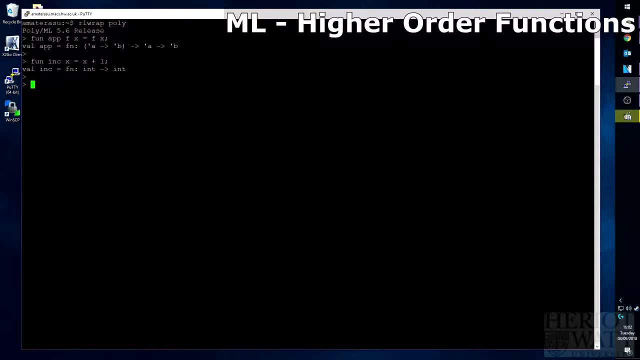 We can now take that function and apply it to the f in the previous function. So if we do app inc, What that's doing is it's storing the function x equals x plus 1 in place of the f in the app function above. 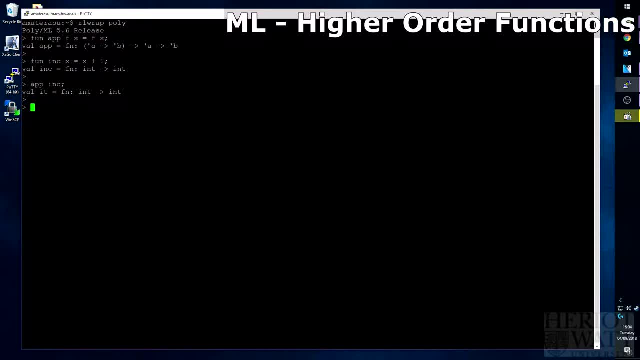 Something to remember when doing partial application is that any information you apply to the function, it will take up the leftmost argument first. So as we've put in the inc function into the app function, it is taking the f place. So if we add in another variable it'll go into the x place. 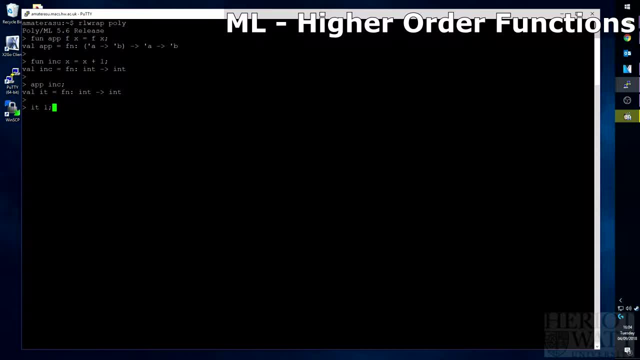 So if we now do it 1,, that'll go into the x, which will then go into the inc function, and it should increment it by 1.. So that is the first function: taking in a function and value and outputting the result. 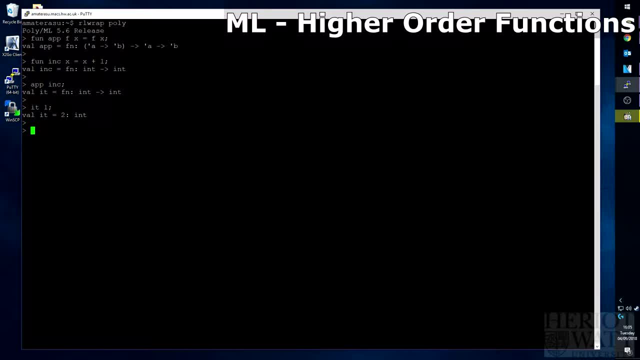 Another way you can use the app function above is simply to specify all the arguments all at once, Instead of using Partial application. So if we did app and then we did inc, which is now in the place of the f, and then do say 3 this time, 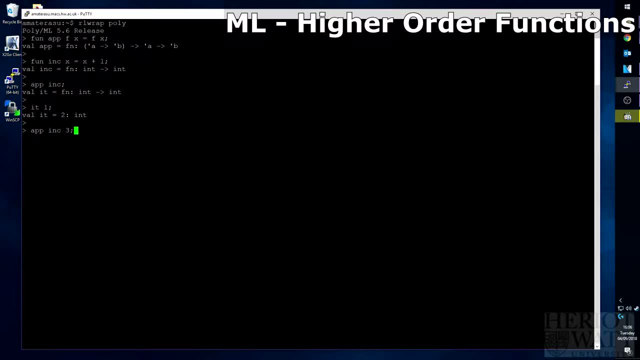 that is the app function taking in an f as inc, and then the x will be the 3. So it'll do all the calculations all at once without resulting to partial application. So this should come up as 4.. This is high Aurora functions in its most basic form: taking a function and inputting it into a different function. 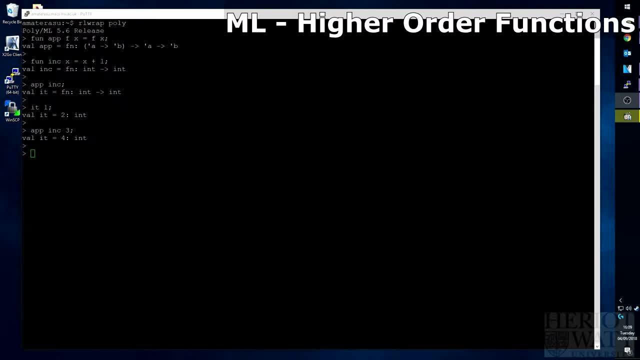 Of course there are restrictions to this, where the function you input must match the type that that function requires as an argument. So if the function requires an int as an argument, you cannot give it a function that outputs a real, but you can give it any function you want which outputs an int. 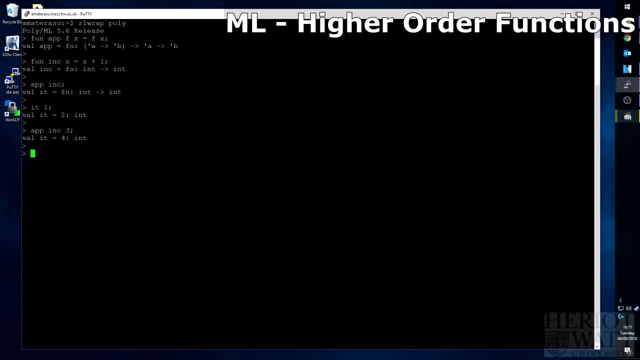 So to show this without getting too in depth into higher order functions, we can take our inc function from before and apply an inc function to it in the place of a value. So we can do inc 1. That is a function being applied into our inc function. 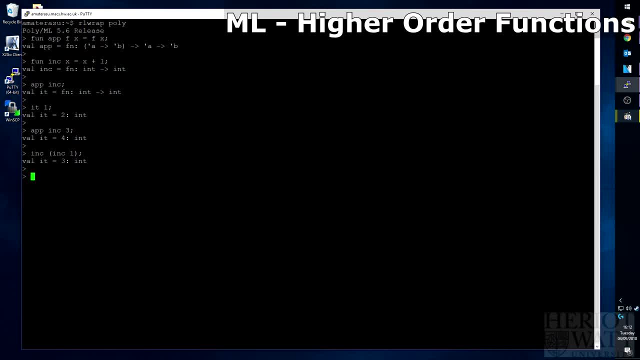 And it works, comes up as 3.. That works because our inc function requires an int as its argument and our inc function outputs an int as well. So now you should have a better understanding of what higher order functions are and what partial application is.